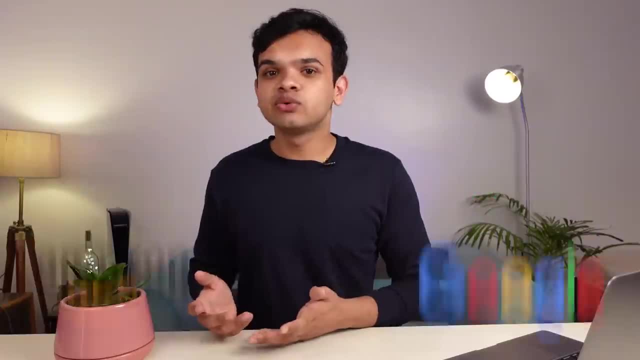 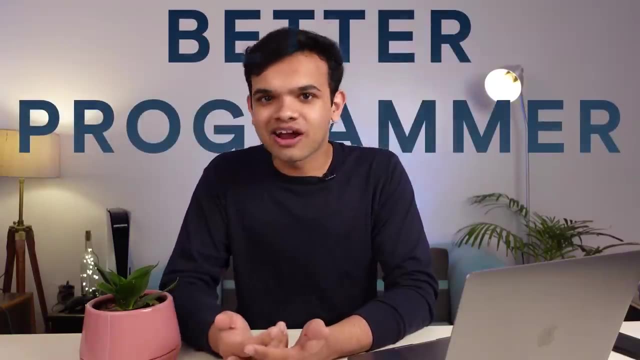 coding questions, and some of these were asked in my Amazon and Google interview, while others I don't think I'll ever see again. I thought, if I was able to solve any problem that was thrown at me, I'll be a much better programmer. and let me tell you the truth: that was far from reality. You don't. 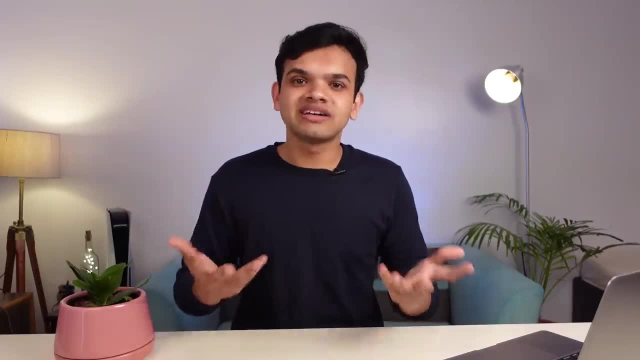 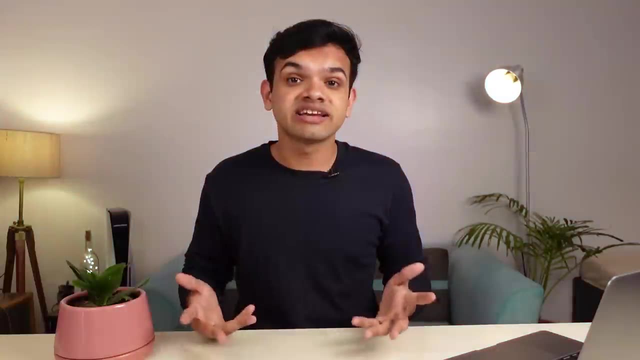 need to end up solving 950 problems and obviously I'm not an expert in this field, but here are the mistakes that I made that you don't have to make, so that you don't have to end up solving 950 questions. So the first thing, and the most important one, is to have a structure You need. 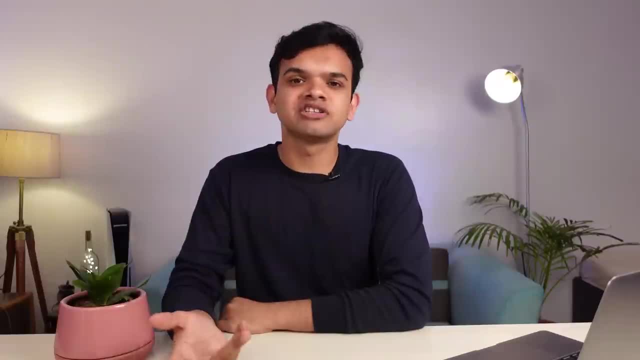 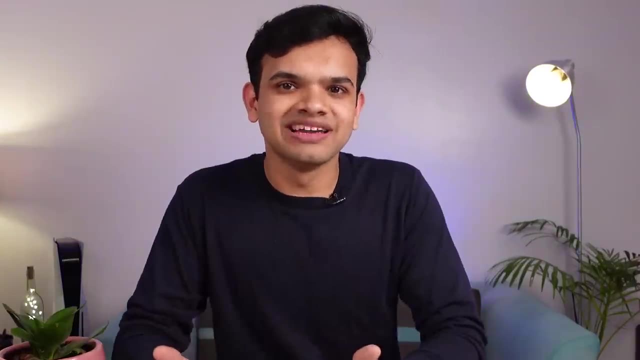 to have some sort of structure when you are trying to learn new things and solve a bunch of questions. I remember when I was starting out, I picked up dynamic programming and graph questions when I wasn't even able to solve array questions properly and I quickly learned that I won't be able to learn. 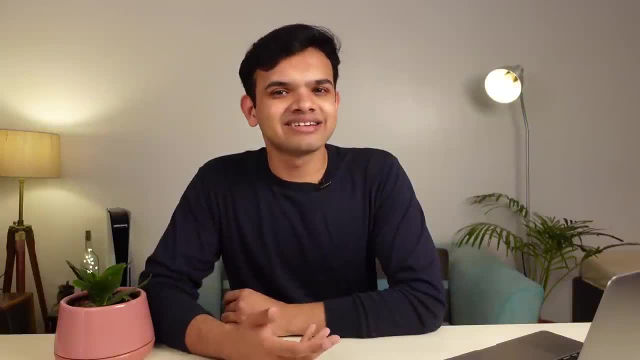 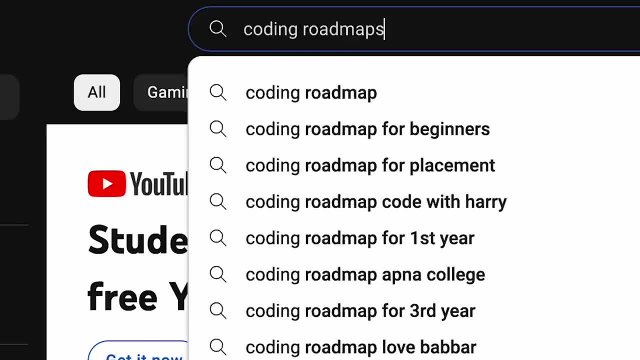 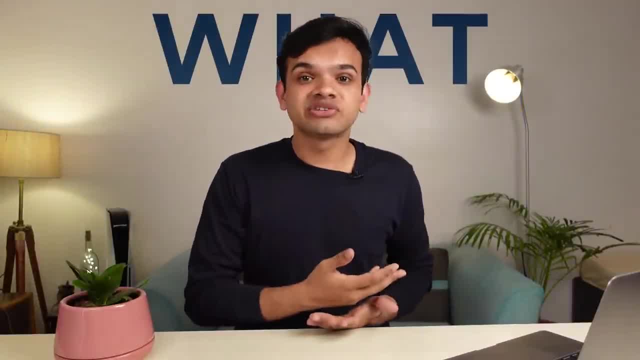 these resources available today, and YouTube wasn't filled with roadmaps, so I had to figure it out on my own. I joined a few paid courses and that really helped me during that time, Like I understood what I needed to study, how I needed to study and what questions were important- Small. 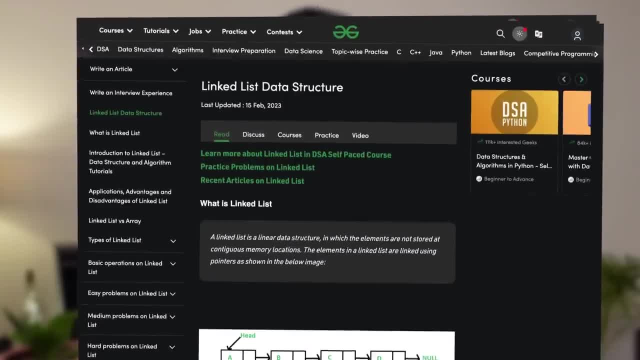 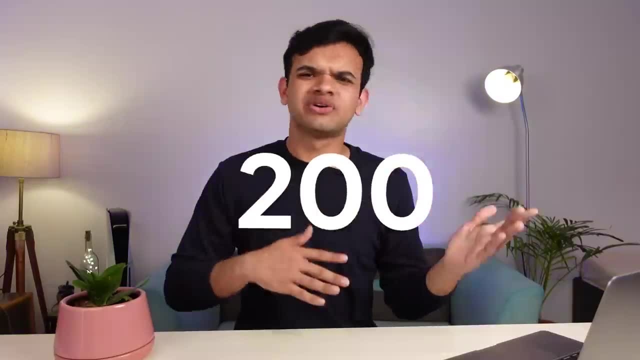 things like how important pointers are before you start trees or linked lists or graphs, stuff like that. Secondly, try to solve questions that are actually asked in interviews instead of just focusing on solving a hundred, two hundred, five hundred questions, And that's not that hard. 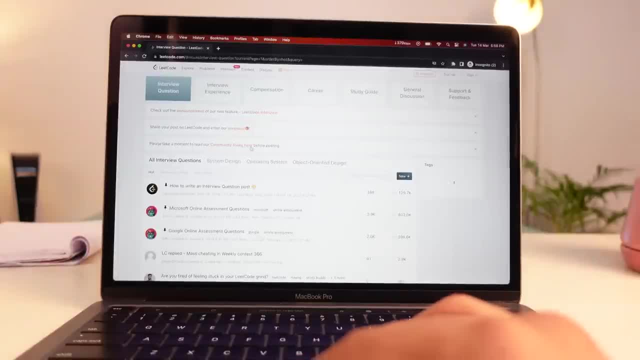 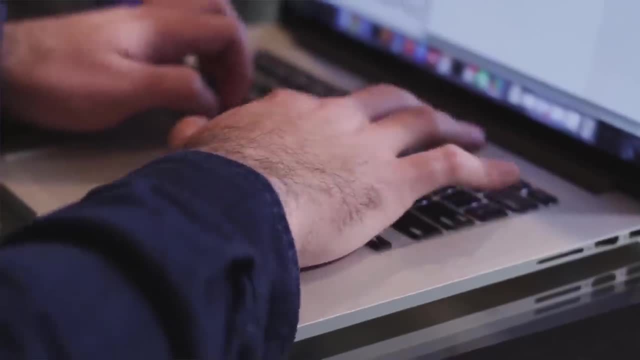 to figure out. You can go on the lead code or the discuss section and read through through company interviews and everything and you'll figure out what questions are being asked right now. Because I made this mistake a lot, Whenever I did a new question, I used to solve 10-15 more questions very similar to this. 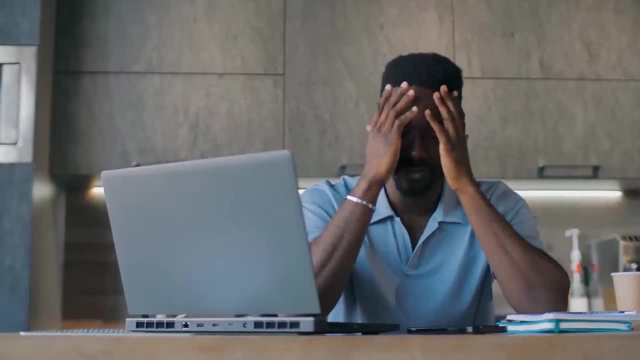 one. Obviously, that increased the number of questions that I've solved, but I didn't really learn anything from those questions and I ended up wasting a lot of time. That brings me to the third point. challenge yourself, but know when to give up. 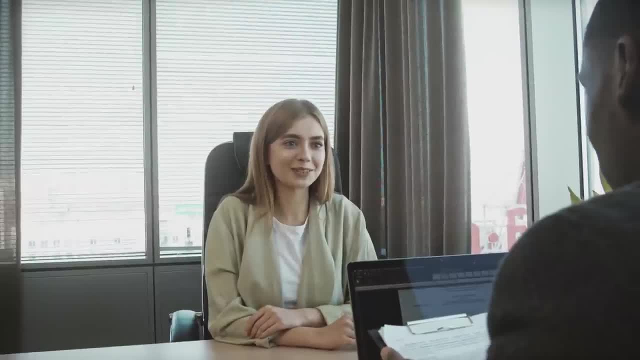 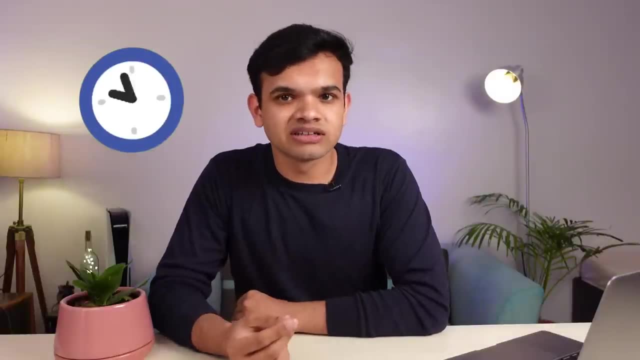 So a typical coding interview is 45 minutes long, even less considering you'll be introducing yourself, talking about the question and a lot more. So you need to prepare yourself to come up with a solution in like 30-45 minutes and, trust me, that is not an easy thing to do. 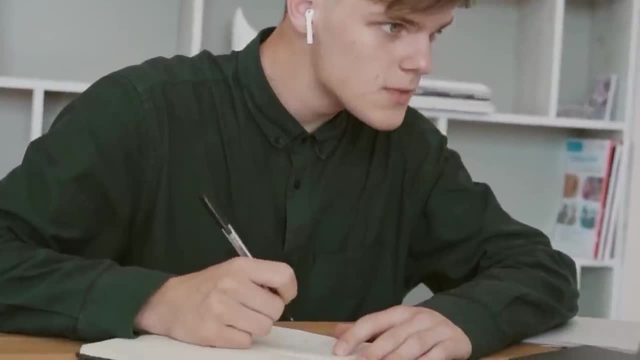 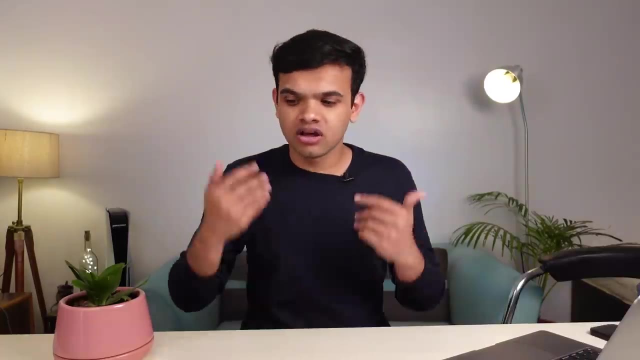 So after some practice, I started to time myself. I only gave myself 30-45 minutes to come up with a solution, and if I didn't have a working code in those 30-45 minutes, I gave up. So usually what should happen is: whenever you see a question, you should have a pretty. 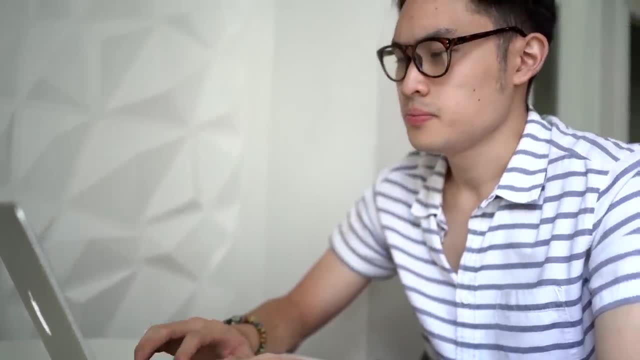 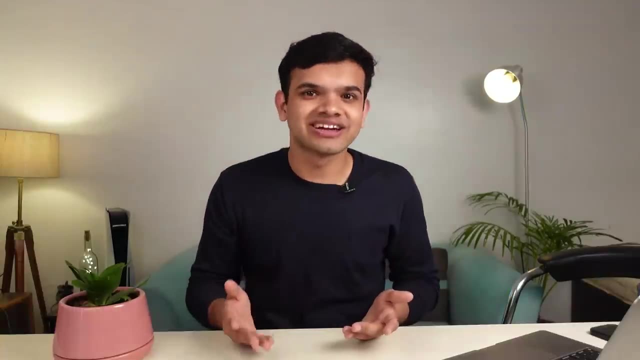 good idea of where this is going in the first few minutes. If I didn't have that idea, I gave up and a lot of people spent hours, even days, on questions. I respect their grind, but that's a lot. I don't have that kind of fun. 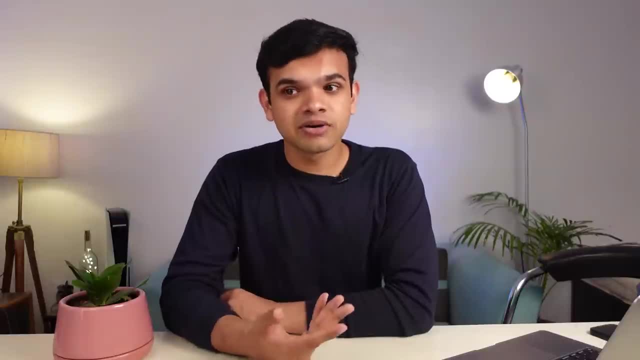 So if you can't come up with a solution in 45 minutes, give up and then go look for a solution, Which brings me to point number 4.. Irrespective of whether I was able to come up with a solution or I was not able to come, 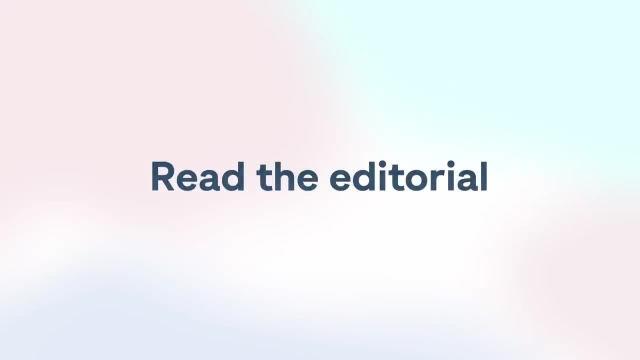 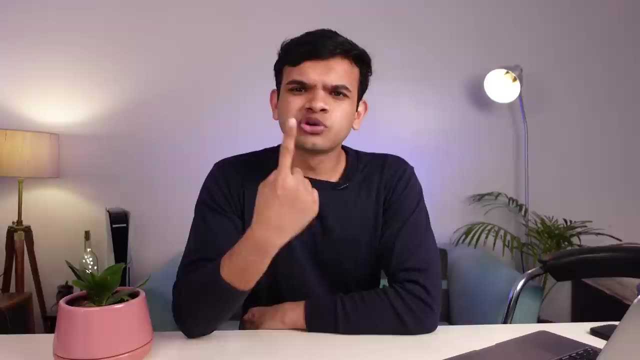 up with a solution. I always went ahead and looked at the editorial or the official solution and not just the most optimized or the best solution. I went through all of them. I used to watch YouTube tutorials. I used to read editorials Because you should know all the ways that question can be solved, because that makes 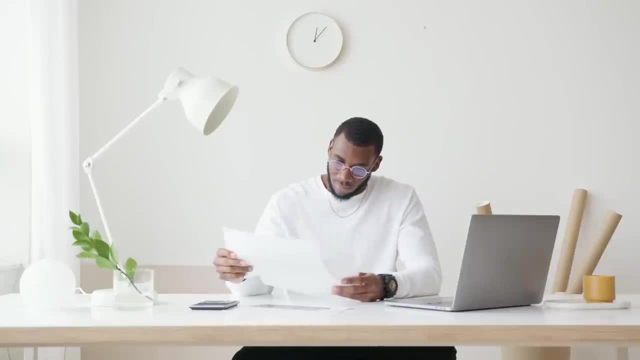 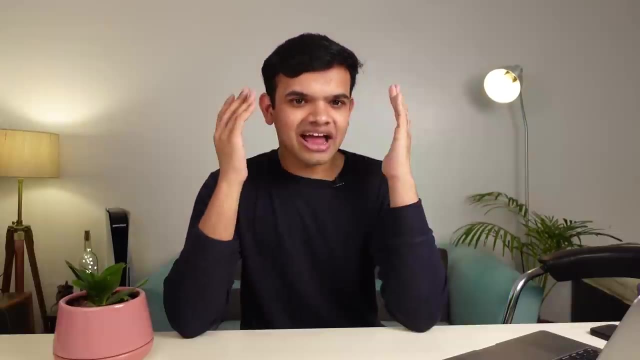 you think about the different ways and how you can use the solution of this question to solve problems. Let's say another question. I have done this a lot. You get introduced to new tricks and techniques and sometimes you look at the solution and think: wait, I could never come up with something like that. 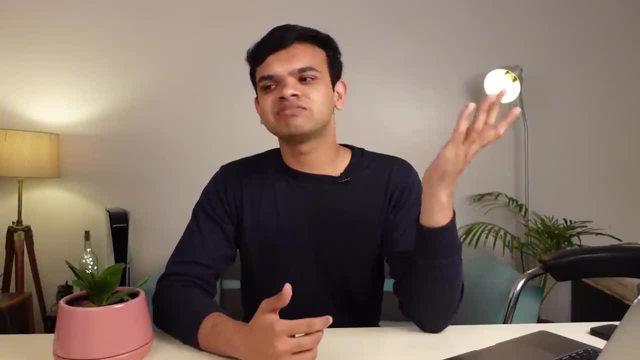 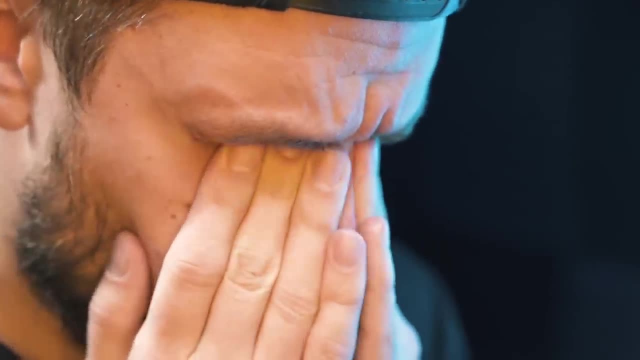 And congrats. you have just learned something new that you will hopefully be using in your next question. Also, try to not learn the solution, because that hasn't worked out ever and I'm pretty sure it won't work out in your case. You'll probably forget half of it, and it will be much better if you understand what's going. 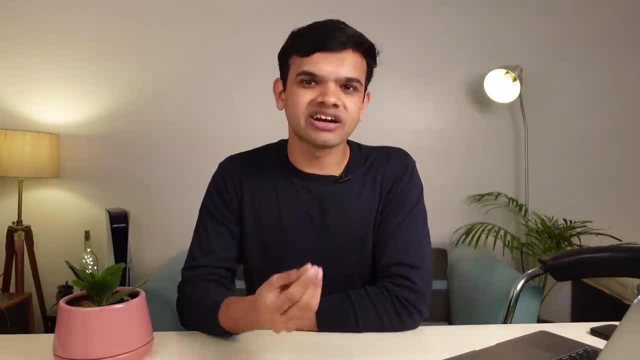 on. This is why I preferred YouTube tutorials over editorials when I was just starting out, And this brings me to my next point. Just understanding the solution is not enough, So I'm going to show you how to solve the problem. Let's start. 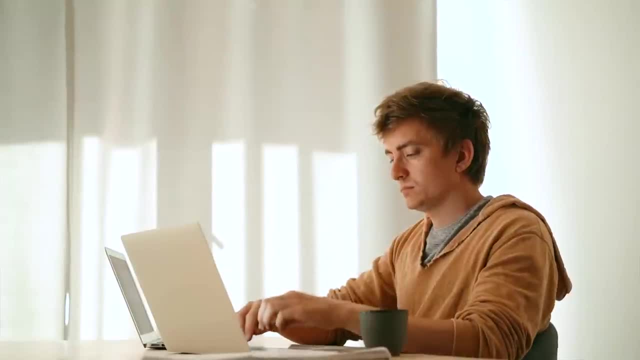 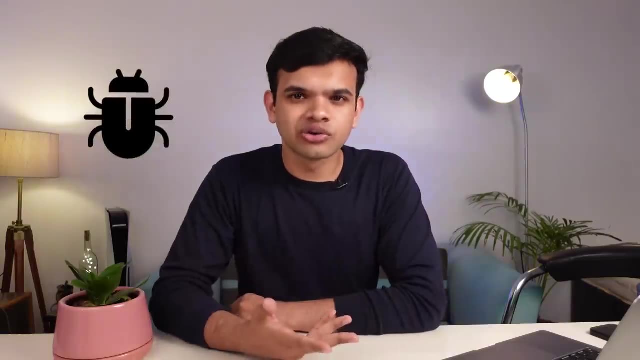 You need to go ahead and code it yourself, Like you need to understand what's going on and then write your own code for that solution and try to summon that. What will happen is you'll make mistakes, you'll add bugs to your code, you'll get stuck. 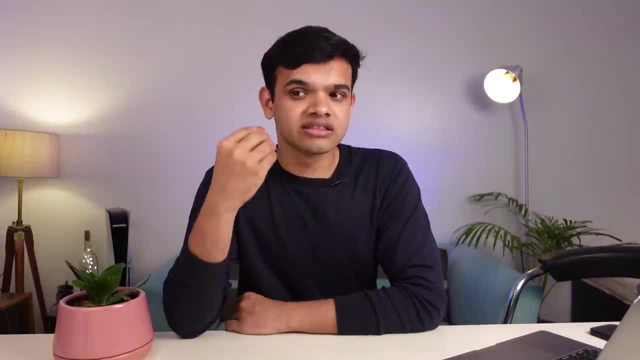 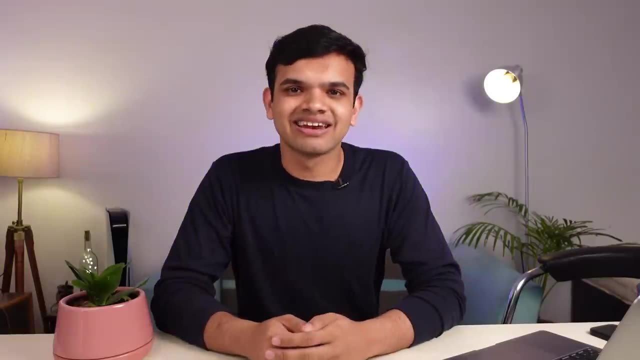 in edge cases, and that's good, because that will help you learn things that you probably wouldn't have learned otherwise. It's better to be stuck right now than in an actual interview And hopefully you don't make the same mistakes again. And lastly, I had this problem a lot. 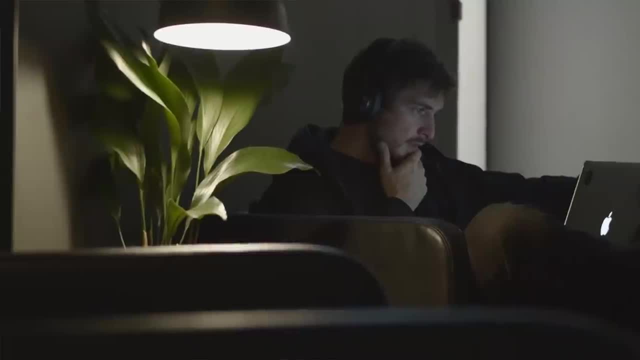 I used to forget a lot of questions when I came back to them in a week or a month, I just couldn't figure out what I did and why I did it. Even my own code didn't make sense to me a lot of times, and this wasn't just me.